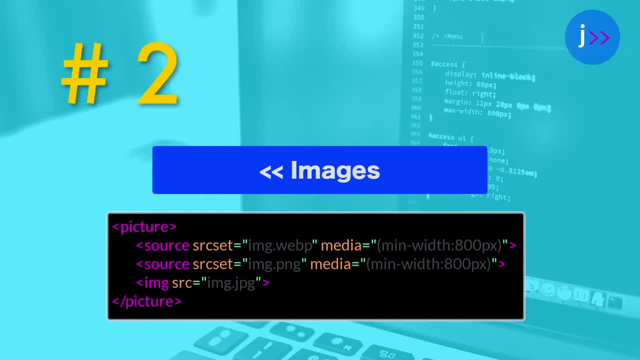 screen pixel densities, and or also use the picture element to allow you to manually add source tags for the browser to pick up which image type to use, based on different device characteristics like portrait versus landscape. If you decide to use the picture element, also make sure that you use an. 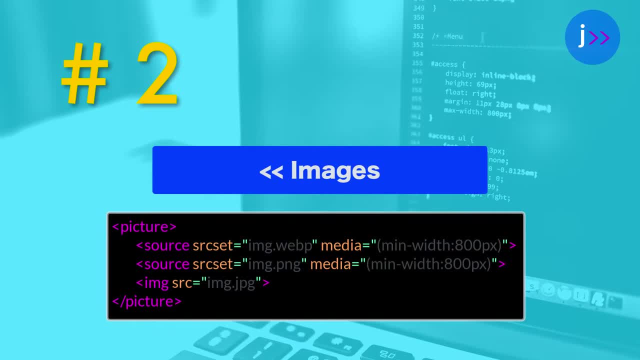 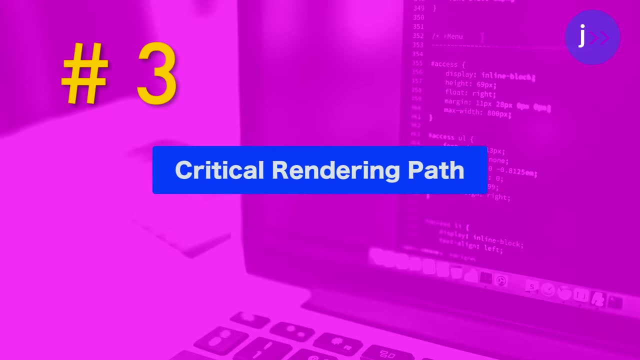 image tag to fall back to, just in case you need to add a new file to use the image tag If you're picture element isn't supported. Tip number three: Prioritize the critical rendering path. The render tree is composed of both the DOM and the CSSOM trees On page load. 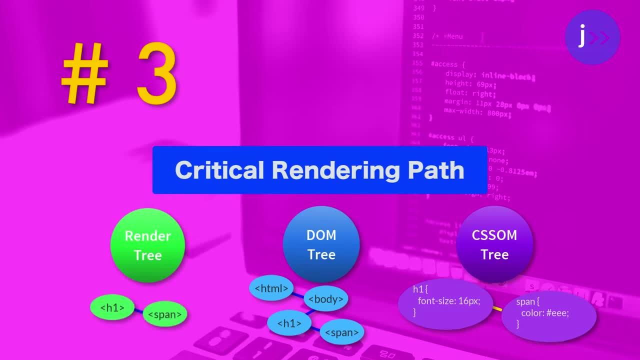 after traversing the DOM to find all of the visible nodes in the DOM tree, the CSSOM styles that go with those nodes are compiled together to create the render tree. Prioritizing only those HTML elements and their associated styles for the initial page load is important to maintaining an 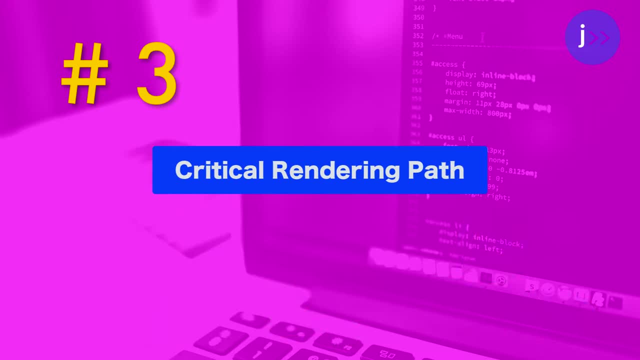 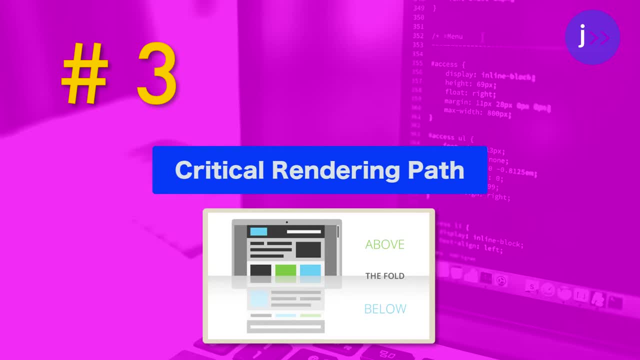 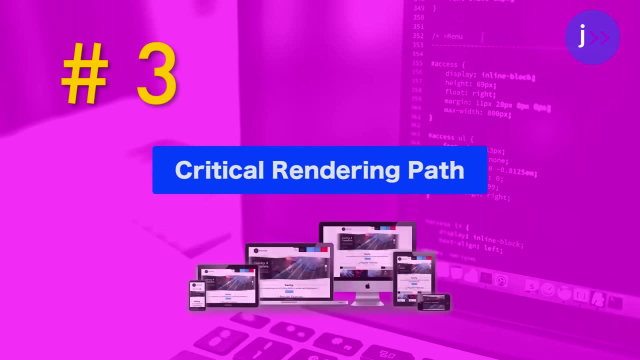 only what would be seen first was critical. However, web pages don't fold and should really be thought of in a fluid and responsive manner within a viewport. If your user decides to say, for instance, flip their device orientation from portrait to landscape, make sure that any 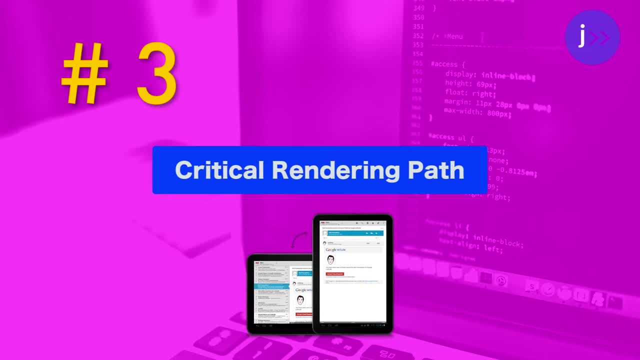 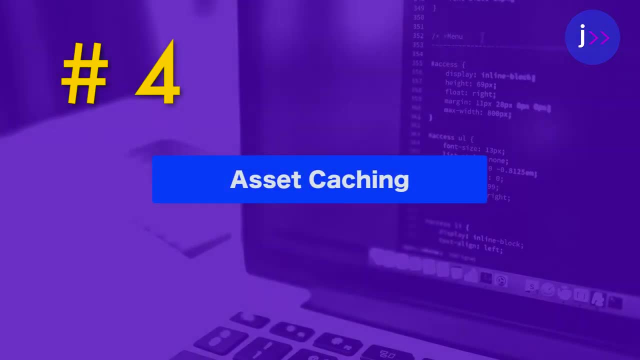 layout changes that occur within the viewport are also considered ahead of time for an optimal user experience. Number four: caching your assets. We talked about CDNs in terms of their benefits with DNS Lookups previously. CDNs also give us a distributed way to cache our assets. close. 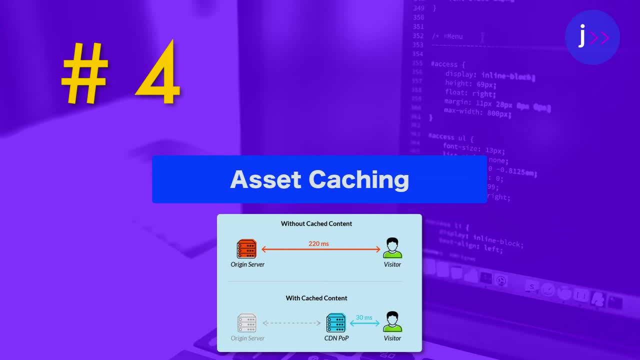 to or in the regions of individual users, so all content and file requests will have a shorter distance to travel and won't bog down your server. This gives you the added benefit of a faster load time for everyone that uses your app. You can customize your caching strategy. 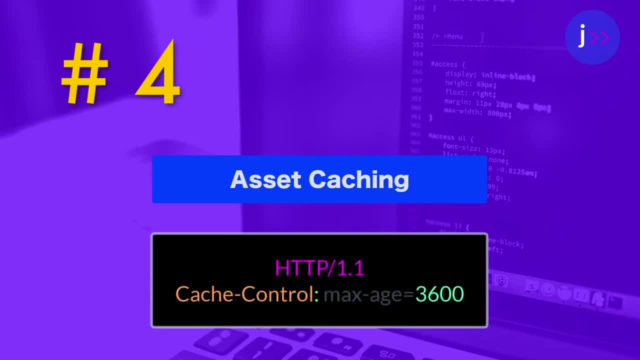 as one size certainly doesn't fit all, with the cache control HTTP header for different types of content and specifying the max age directive to the duration of time you'd like to keep a file in the cache before it expires and a new one is requested. Leveraging use of a user's local cache. 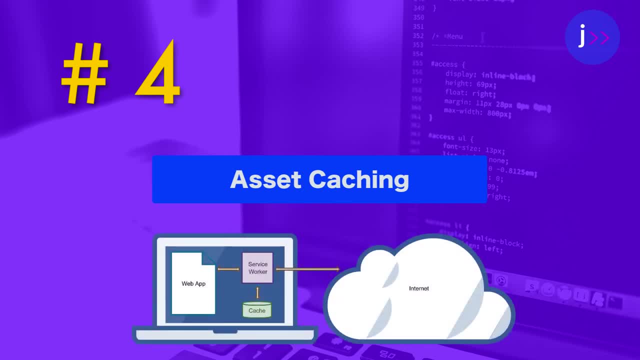 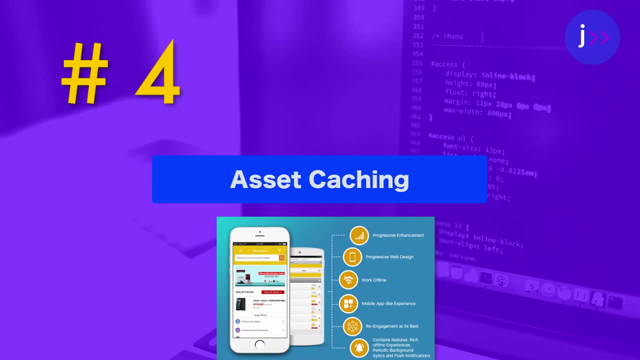 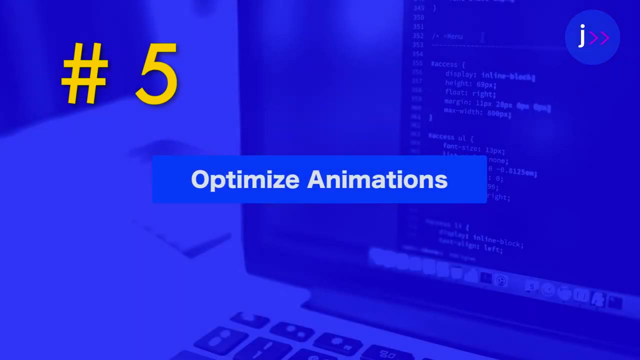 on their browser or device so that your app loads instantly, is another caching strategy that proves especially useful in the case of progressive web apps, or PWAs. This allows your site to be available even if the user is offline. Number five: optimize your animations. 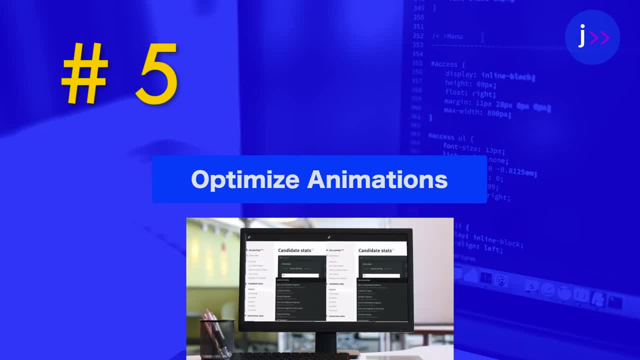 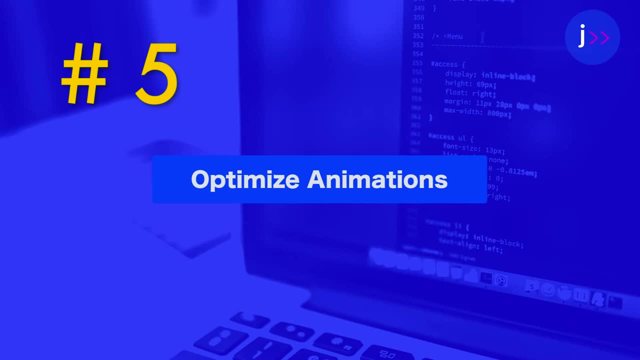 To make sure you minimize jank with your web animations and avoid a significant slowdown throughout your app's front end experience. you wanna make sure that you give an element's CSS selectors a heads-up as to what properties will be animated. You can do this. 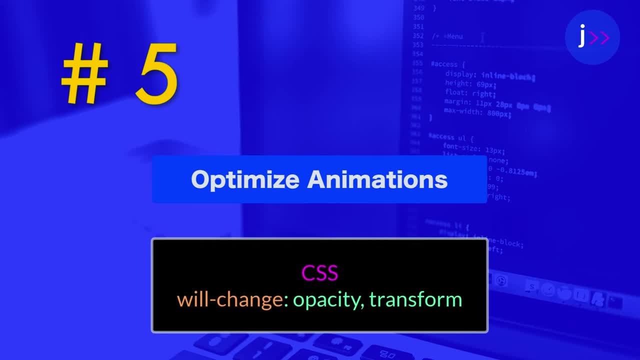 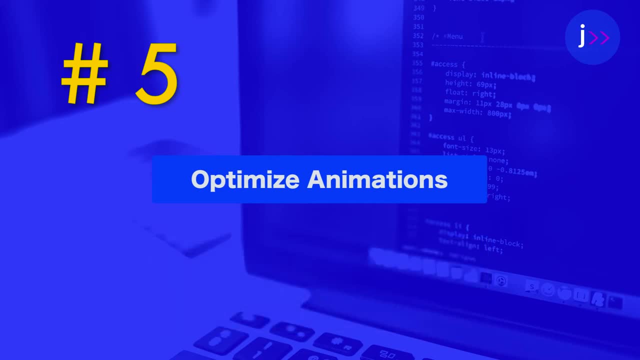 by making use of the will change CSS property and setting it to the value of the property that will change once that animation is triggered. Another way to optimize your animations is to avoid using set interval or set time out and to opt for the requestAnimationFrame method. 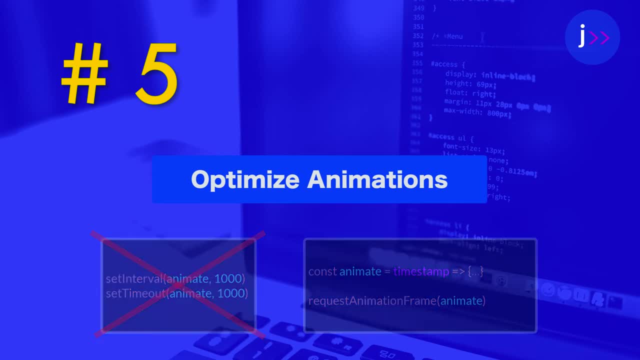 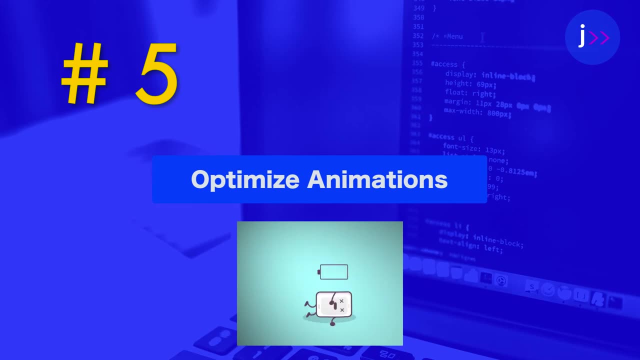 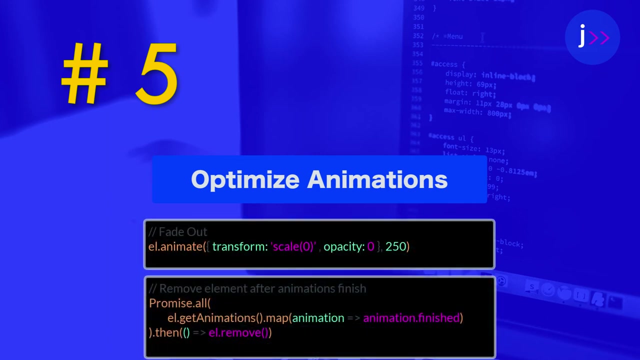 This will avoid running your animations when a user's tab isn't visible and save a user's battery life and save render time prior to the next repaint. When animating with JavaScript, use of the Web Animations API can also be a huge performance saver and give you more granular control over your complex animations. 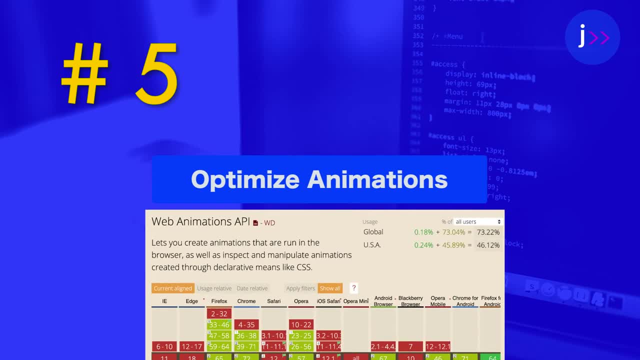 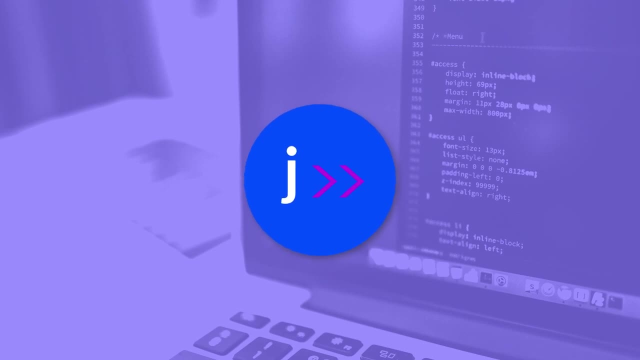 At the time of recording this video, the Web Animations API has support in around 75% of global browsers and close to 50% of US browsers, so a polyfill is most likely necessary if you want to boost those numbers. Check the description for more links to dive into any of the topics covered here in more. 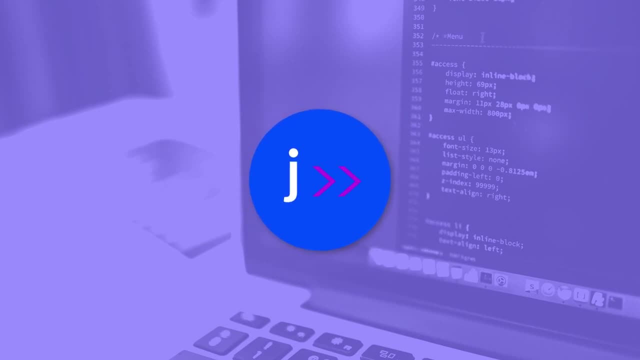 depth. If you enjoyed the video, give it a like and subscribe for more awesome content, and please leave a comment as to what you'd like to see me cover next. Stay golden.